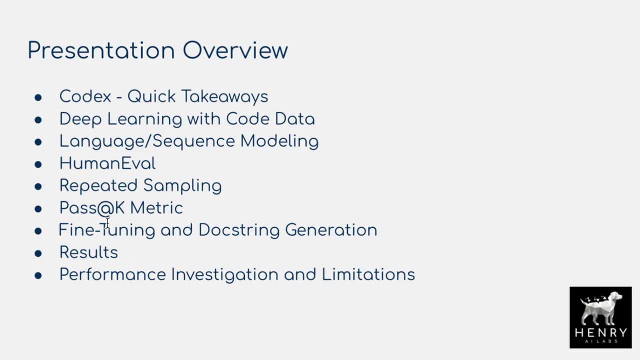 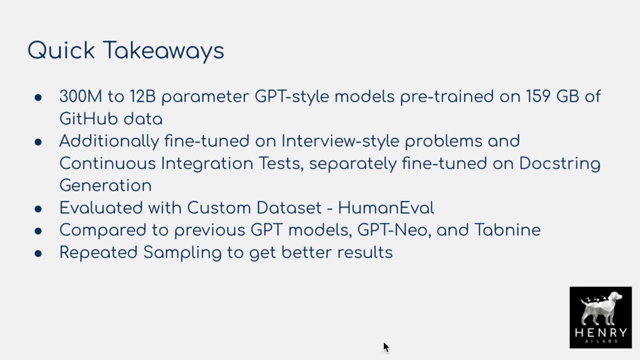 at the fine tuning data sets they designed from the code forces, competitive programming, interview style questions, as well as continuous integration tests from these public GitHub repositories, which are pretty interesting, and then a docstring generation. So they reformulate the problem. So instead of going docstring function signature implementation, function signature implementation than docstring so rearrange the fine-tuning data set like that so that the model can then be used to write like natural language explanations of the code in that kind of left to right autoregressive gpt style i will look at some results and different things they take apart and then the performance investigation broader impact list they state as well as limitations like you know particularly where the docstring generation fails so here are some quick takeaways from the paper they train different scales going from 300 million parameters up to a pretty large 12 billion parameter model is a massive model it's about the size of the t5 model it's not quite gpt3 scale but 12 billion parameters still a pretty massive model so it's pre-trained on 159 gigabytes of github data later in the video we'll take apart exactly how big 159 gigabytes of you know code data really is it's additionally fine-tuned on these interview style problems and continuous integration tests but again this fine-tuning is more like a domain 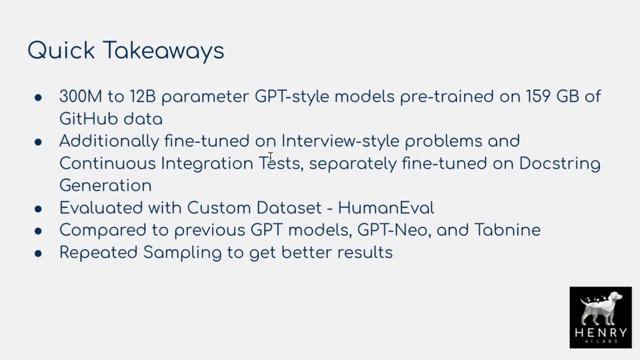 supervision because it's still doing this likelihood minimization with this sequence the sequence generation task is still trying to you know auto aggressively go left to right and 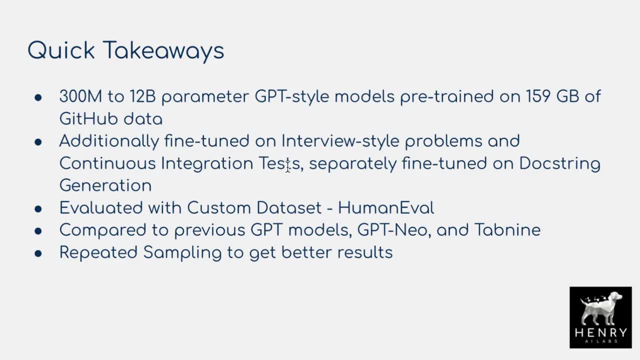 predict the correct token has been masked out always at the rightmost part of the sequence but now the domain is more interview style problems in these tests which are better aligned 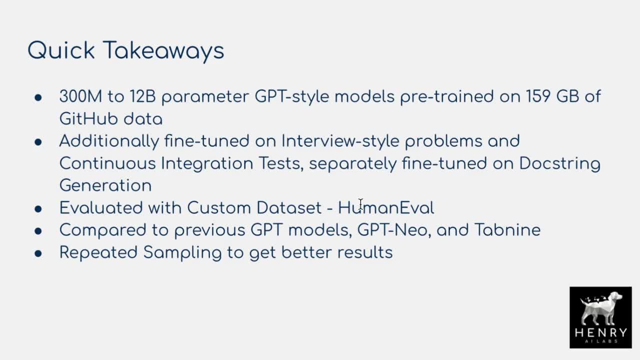 for then evaluating it on say the apps benchmark or this human eval custom data set so they could construct a custom data set it's not really that big it's 164 examples with an average of eight 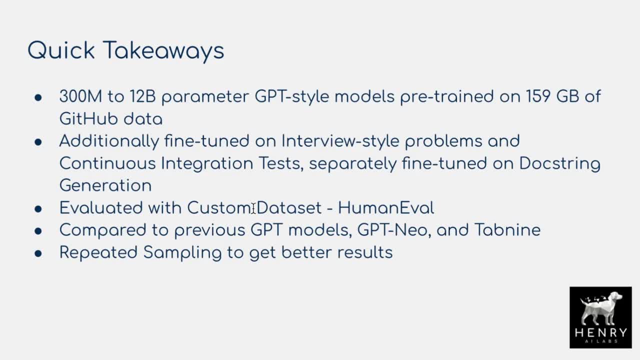 about eight test cases it's not really a massive data set but they use this to evaluate the model 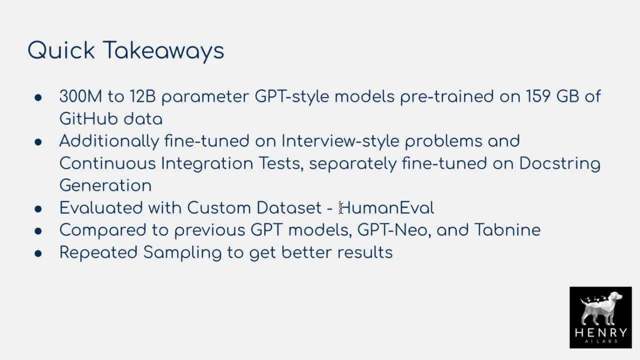 and then you know report the when reporting the percentage pass this is what they're talking about they compare it with previous gpt models like how well gpt3 would do its transfer into this as well as the eluther ai gpt neo model 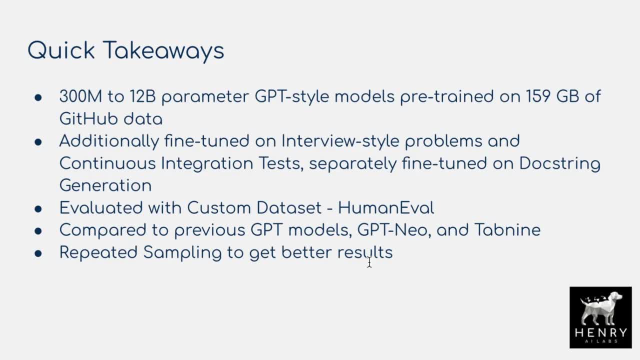 and then also the tab 9 autocomplete tool and then the big takeaway from this is using repeated sampling to get better results so instead of just doing one greedy decoding of the generation tree 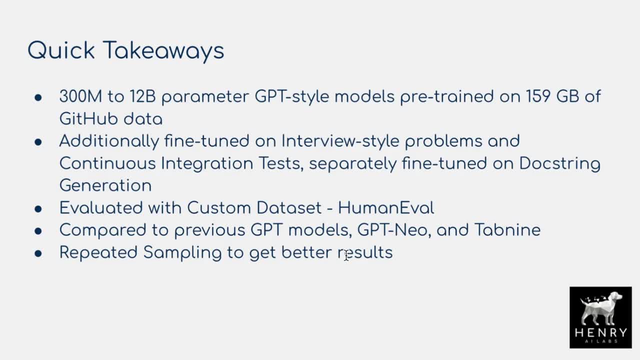 you can sample say 100 of these with you know different values for the temperature and you know how you traverse the tree and this really helps and it's really useful for say code where you have this ground truth evaluation does it pass the unit test compared to where to say text 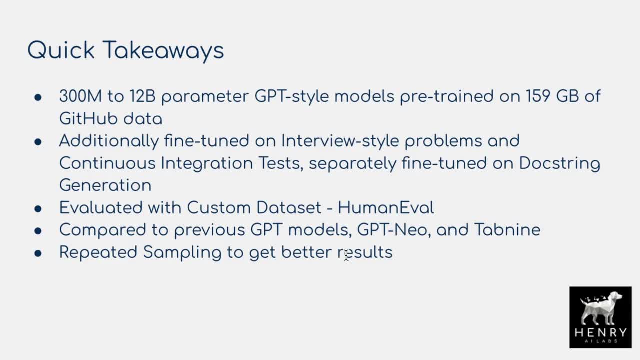 generation if you just do all these different samples you now just have a bunch of samples and it's hard to really pick which one you know you pick which one through something like greedy decoding or as described say the mean log probability of the traverse through the tree 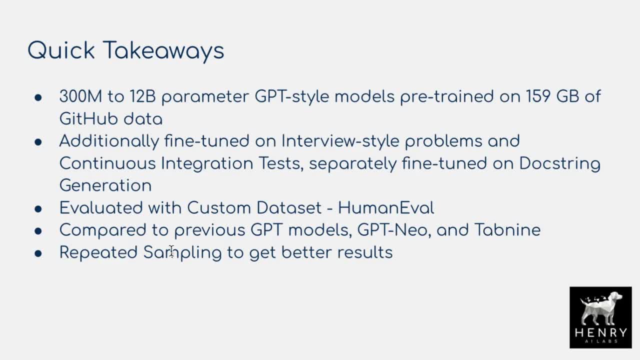 these different ideas so repeated sampling works particularly well for this application setting where you're trying to pass these unit tests so you have this kind of like ground truth evaluation of different generations evaluating the output of these kind of esoteric domains like image 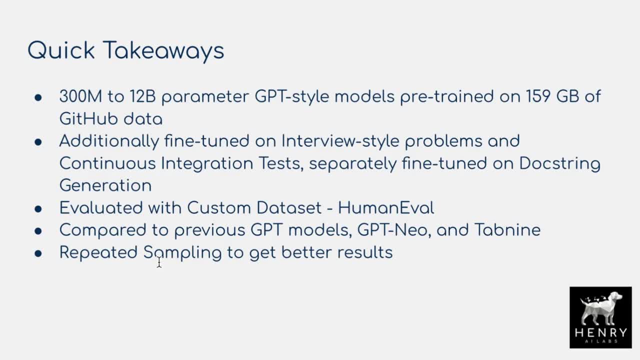 generation and text generation is an active area of research it's hard to say that you know this style gan model versus the big gan self-attention gan you know this these generated images are much better because you don't have this kind of automated metric and again there's a lot of research that 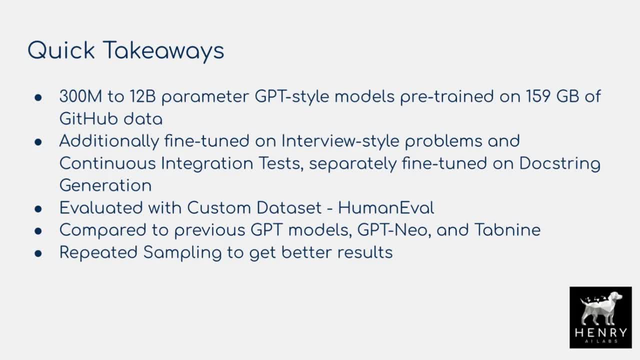 does this and it's different from passing these unit tests which we'll talk about more later in the video so if you're curious about what these programming problems look like here's a quick 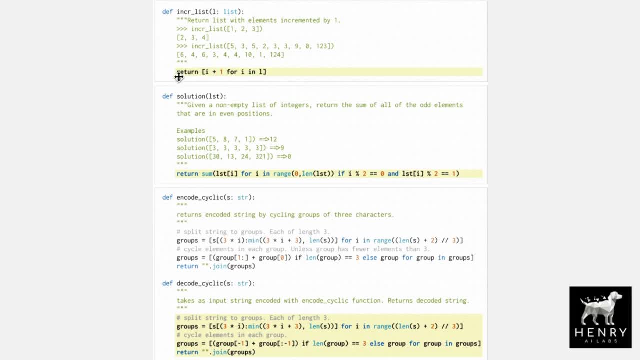 image that shows exactly the programming style problems the code that the model is being trained to generate so say you have the function signature increment the list it takes in as input argument a then you have this doc string in this case providing examples of what the function is 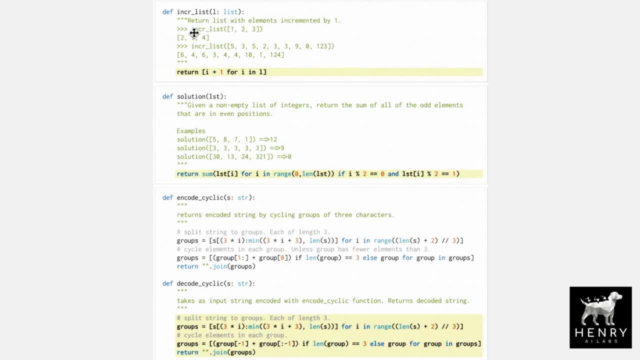 supposed to do so return list with elements incremented by one showing that if you pass in as this list argument one two three it turns it into two three four then another function def 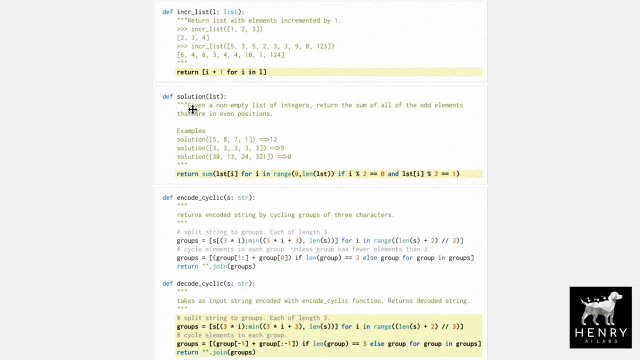 solution list so you get nothing from the function signature in this case but the doc string is telling you what the what that you're supposed to implement in the resulting python code so the model will learn to generate these functions that satisfy these doc strings and so on and then 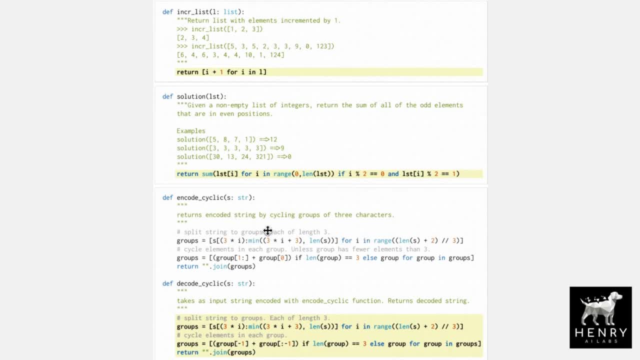 when you have these test cases you give it the function signature the doc string and then you know it generates the code and then you have these unit tests to evaluate say the edge cases the average cases and these kind of like leak code hacker rank style evaluations of these algorithms 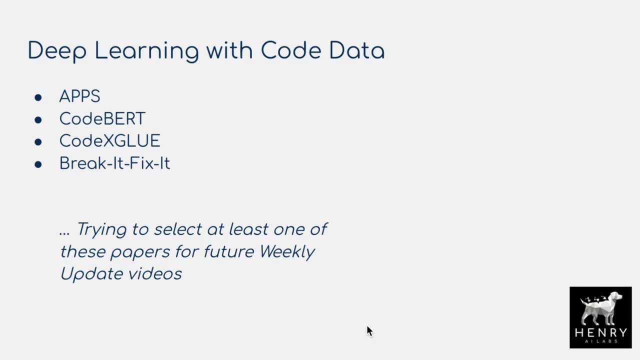 so there's a little bit of a background on deep learning with code data there are these different papers that are exploring using code and programming languages as the data set for these 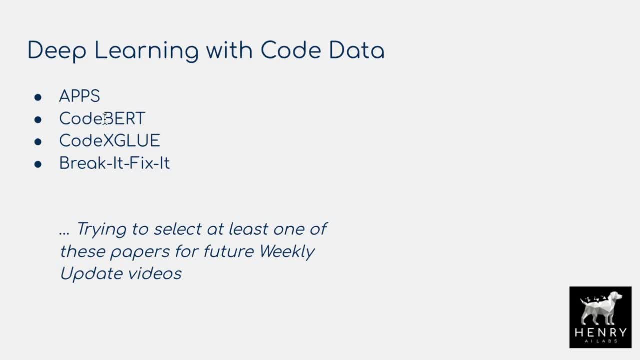 tasks so code bird is also doing this kind of like electra style language modeling with say java javascript python code codex glue is a collection of say what kind of supervised learning tasks 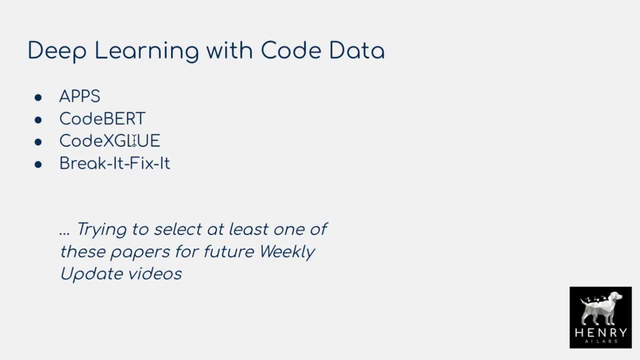 that we can do with code data and then codex glue benchmark that said we have text classification natural language inference duplicate question detection trying to unify all these different 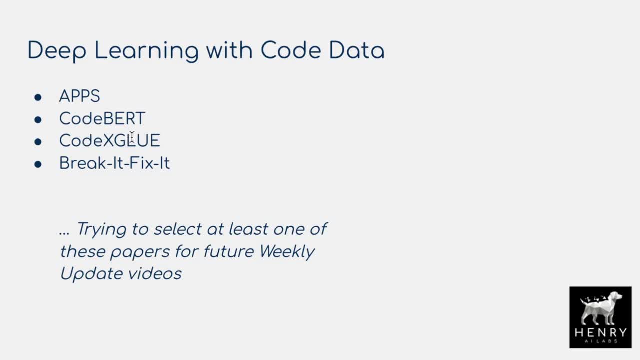 supervised learning tasks we can think of in the natural language domain codex glue is trying to 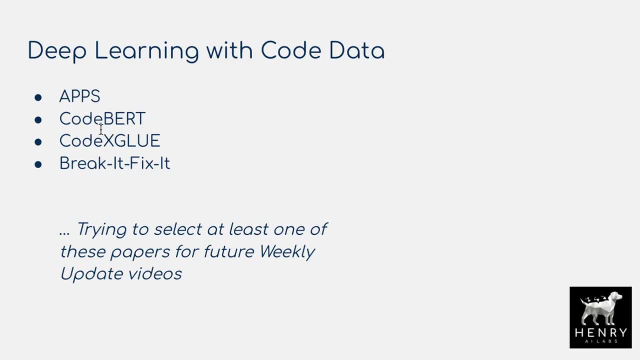 do that with code and also going bridging these domains between text code code only text only so you know integrating say natural language descriptions of code with the doc strings and so on with these kind of tasks we can do with code data and then just recent paper i'm trying to 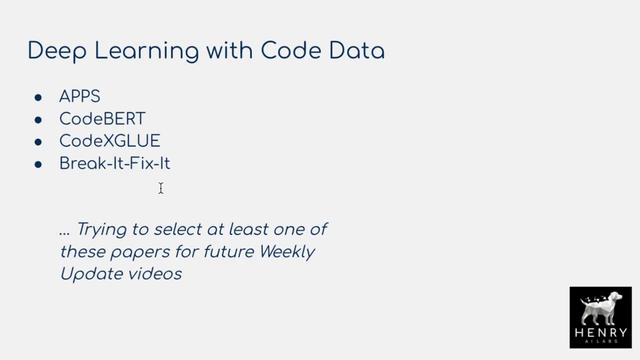 select more of these in the weekly update videos break it fix it is looking at this semantic errors of your code so instead of having to take that frustrating debugging error and paste it into google potentially solutions that could you know fix your code for you and pass it through the compiler so really interesting domain accelerating really quickly and should be this really 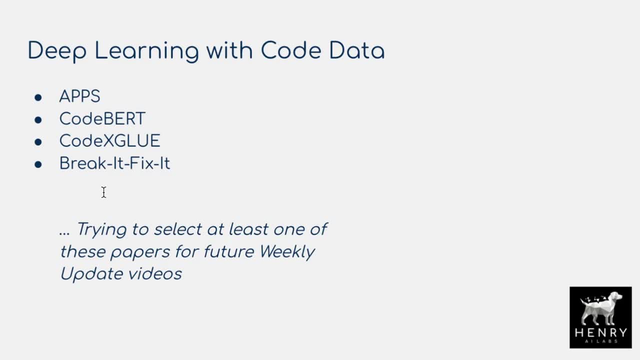 interesting kind of augmented intelligence meta tool for deep learning researchers and programmers that help with these kind of workflows and these kind of problems so the bigger trend at play here 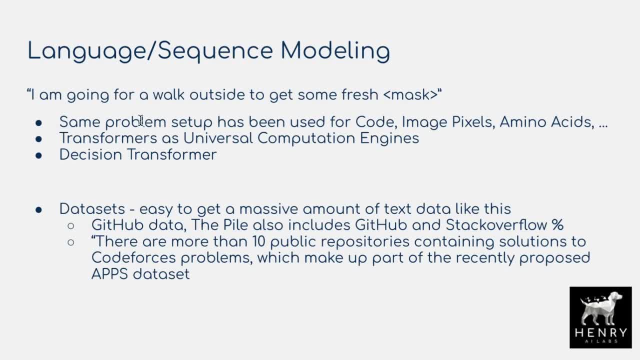 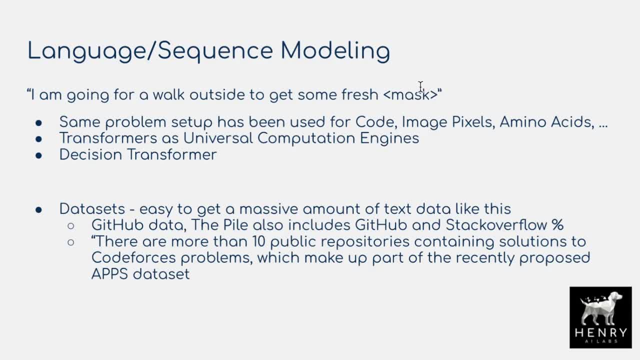 sequence so i'm going for a walk outside to get some fresh and then say predict air compared to a vocabulary distribution that could include like tiger or zoo or car whatever there could be this 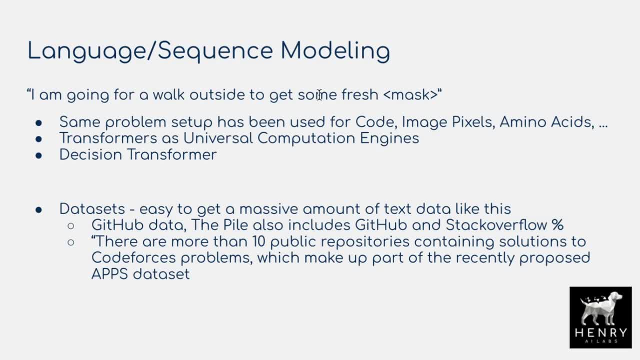 big vocabulary distribution it has to predict the master token and you do that at a massive scale the data can automatically label itself as in self-supervised learning and it's proven to work 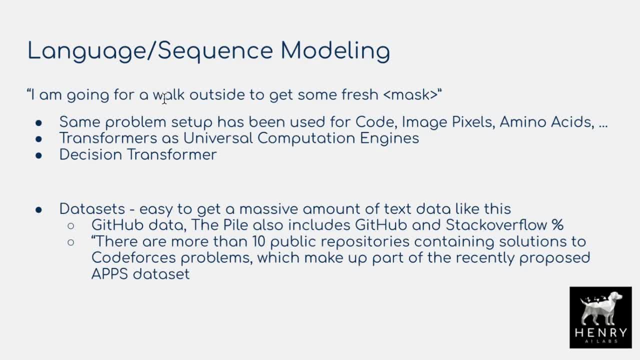 well so they're scaling this up to other domains there's a huge research interest in deep learning taking this to code image pixels amino acids moving this idea of this sequence modeling task into other problems so transformers is universal computation engines is looking at how well these pre-trained transformers can do image classification just you know treating the pixels as a sequence of 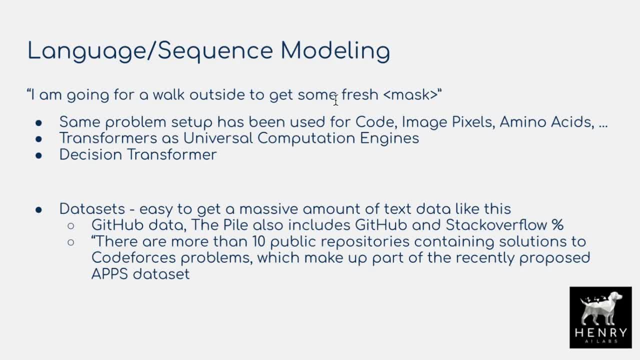 image generation just going auto-regressively left to right but it's very interesting and especially for code amino acids and so on so 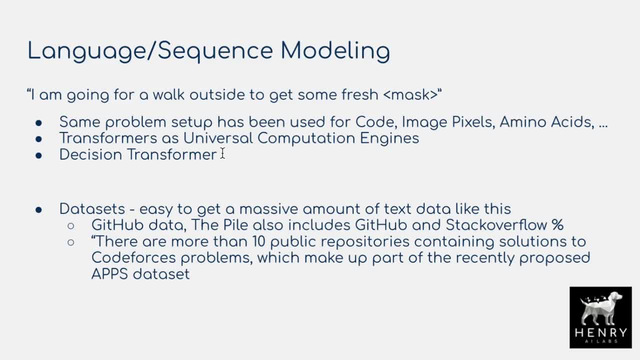 the decision transformer is another really exciting paper that shows say when you have these reinforced learning problems you also have this sequence problem reinforced learning you're 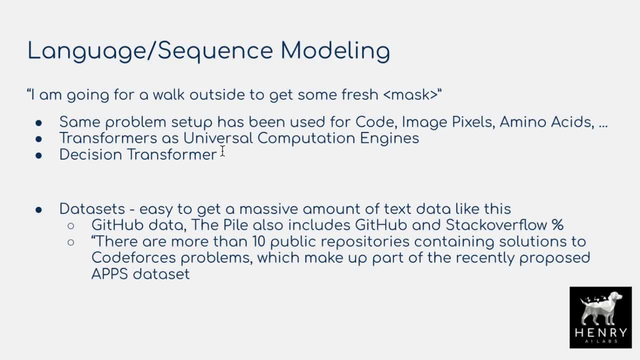 predicting a set of actions given a set of input states you can also look at this as a sequence learning modeling problem where you maybe have more of this sparse reward as in the reinforced learning setting but they show how you know the transformer this sequence modeling approach by modeling this you know sequence of state action trajectories into some reward is a really 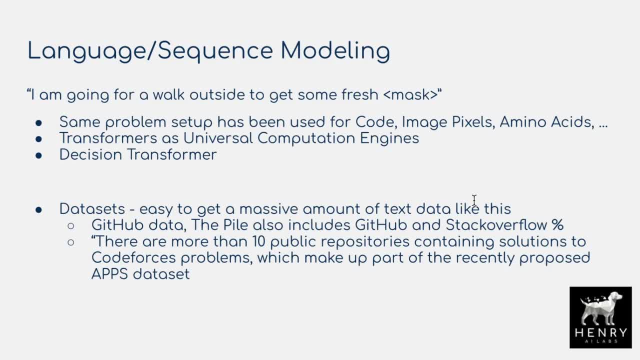 successful framework so we have these data sets it's really easy to get a massive amount of text gets finally we have Seite campo data and dataset for example this first one you have the 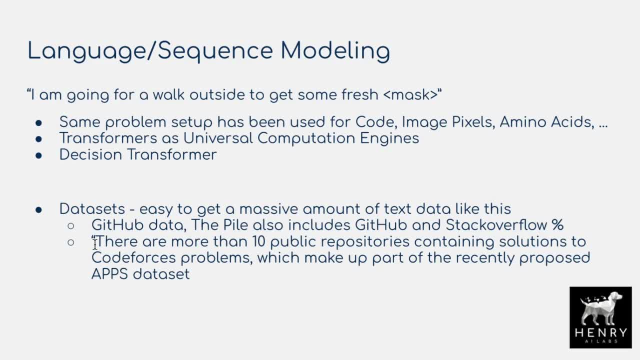 overdraft github data a dataset from elutherai the pile it also includes a percentage of github and stack overflow data and as they mentioned in their in their paper describing the github dataset that's used to train code x there are more than 10 public repositories containing solutions to the code 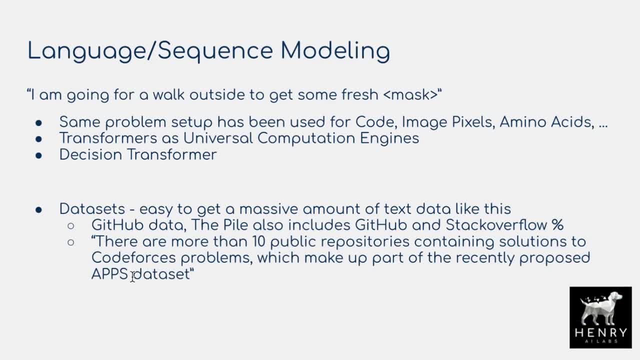 forces problems these are the apps benchmarks this is why they have to construct this human eval benchmark and they can't just report apps because they've seen that data in the training set so this article will be linked in the notion page of this overall ai weekly update series this is a blog post so there are several abilities that we've found and feel worthy of this particular Social Testing multi-page as well as 10 products that we bought or that are Señora's offer is also a great tool in terms of 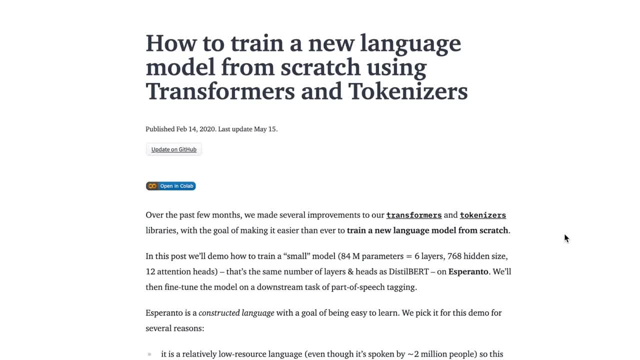 post from Hugging Face showing you how to train a new language model from scratch using transformers and tokenizers, referring to the Hugging Face transformers and Hugging Face tokenizers library. 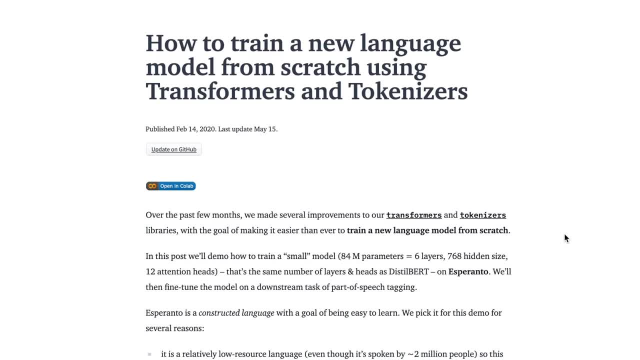 So with this tutorial, you can train a custom tokenizer for whatever, say you have a distribution mismatch, particularly in the code setting, you have this different save you in code white space 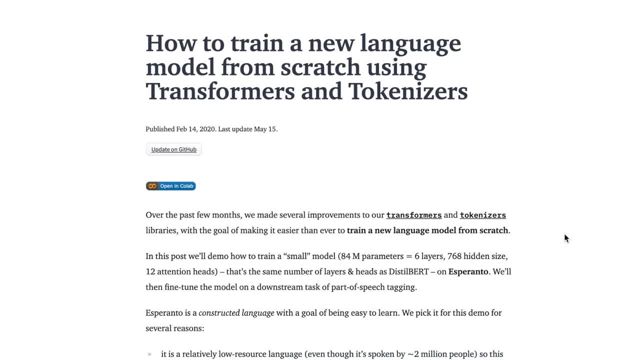 as they describe later in the paper. This is, you know, super inefficient and so on. So this blog 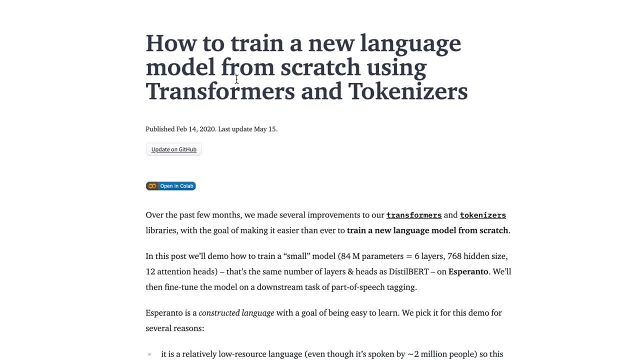 of sequence data domain and use the Hugging Face library to deal with this. So once we've trained these auto-aggressive text generation models, we need some way of evaluating them. And it's hard 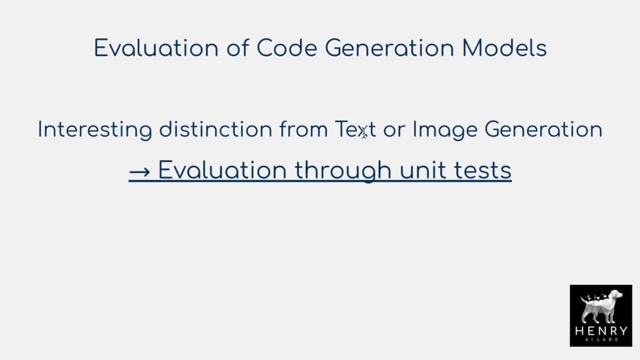 to evaluate these text or image generation models. So say you have a text model like a chatbot or something that writes like a story or a poem or something, it's hard to have just like this 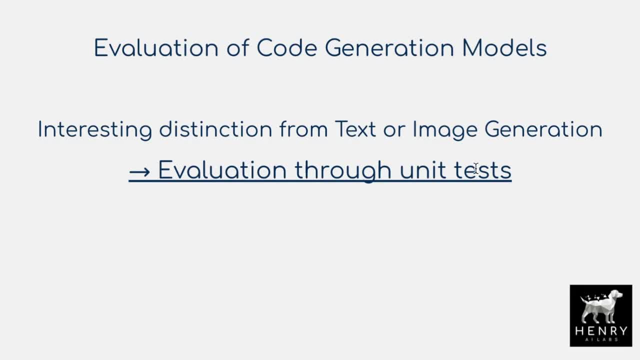 concrete evaluation like you have with these unit tests. So with code generation, you have these unit tests. And I think that's a really interesting and exciting component of this because it's difficult to automatically evaluate text or image generation. 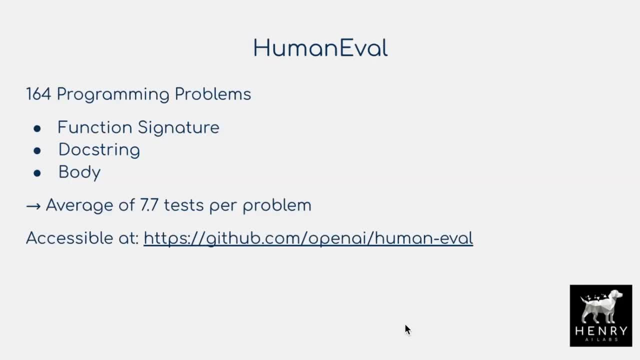 Compared to these unit tests. So in order to do that, the authors manually construct this dataset human eval that is linked in this GitHub repository that has 164 programming problems with 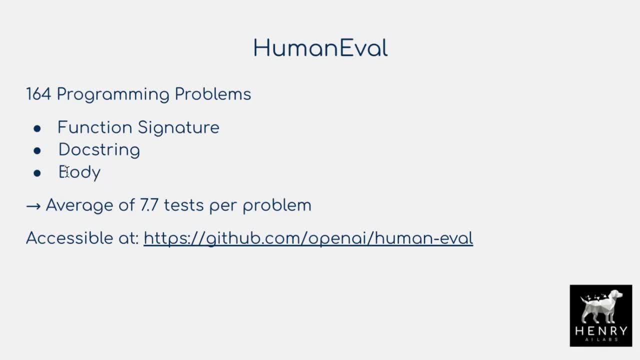 a function signature, a doc string and a body for the ground truth, function implementation, and an average of 7.7 test cases per problem. And this is used to evaluate the different 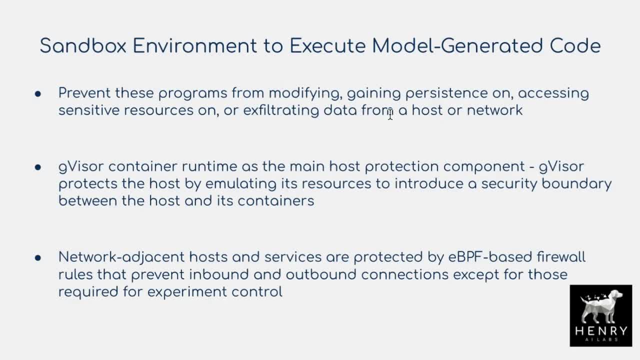 code generation models. So then another interesting detail of, you know, how they're overall constructing these experiments is they have this sandbox environment where they can execute the model generated code, and describe how they use this code generation model to 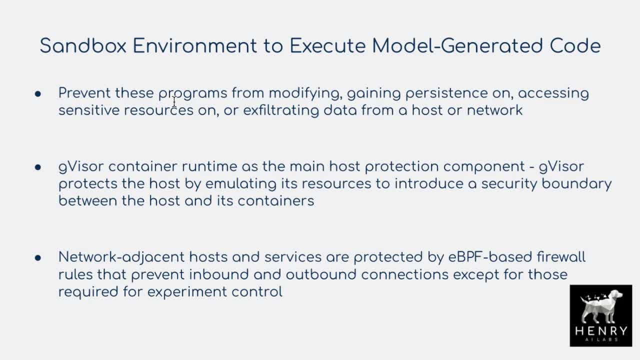 to, you know, avoid these programs that could kind of hack the open AI system and extract data, you know, all these different ideas, and they use this G five visor container runtime, maybe an interesting 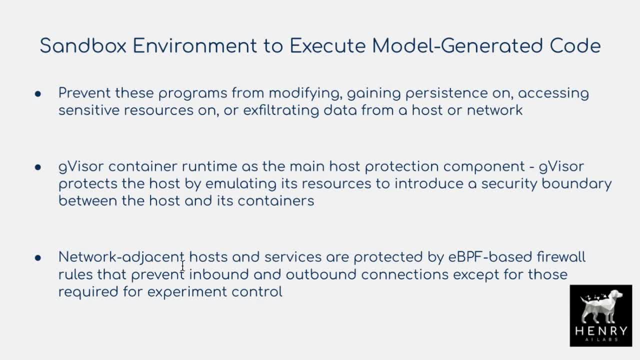 detail for someone looking to experiment with this and, you know, have these runtimes that you're doing, you know, supervise, maybe you have like a reinforced learning environment where it has this 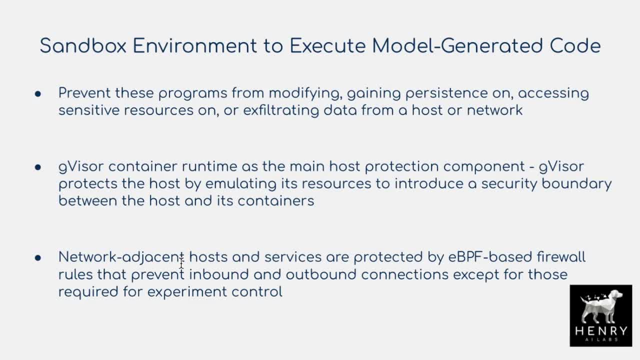 sparse signal, and you need these kind of sandboxes to execute code, a very interesting idea of thinking about how these experiments are designed, and a really controlled setting for experimenting with these kinds of models. 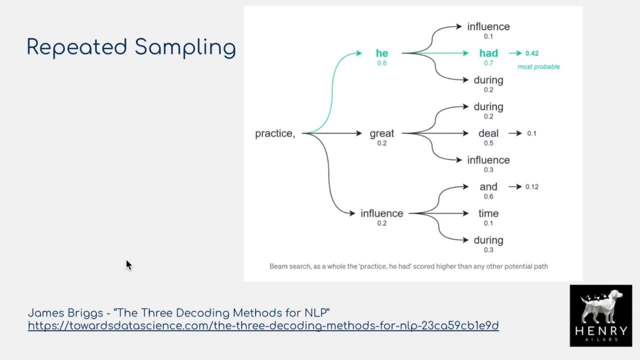 So the real novelty behind this codex paper is this idea of repeated sampling. And again, this works so well, because you have this concrete unit test evaluation. So you can generate 100 different samples, and then 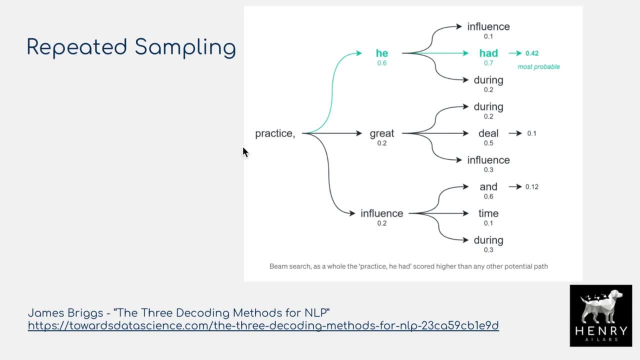 just filter them based on the ones that pass the unit tests. So when you have language generation, or you have this kind of, you know, probabilistic model that is filling out the mass token in the sequence, it has these different probability densities on different continuations of the 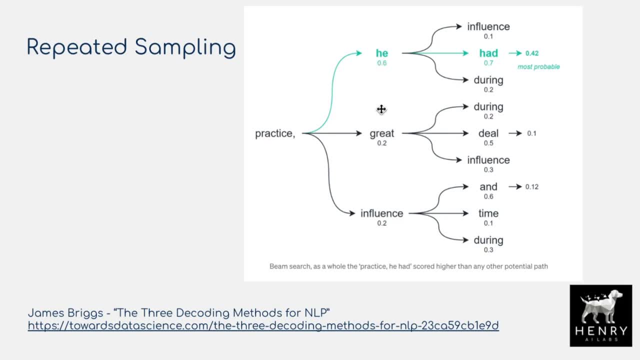 sequence. So in this example, he is given 60% probability grade 20% and influence 20% as a continuation of the sequence. 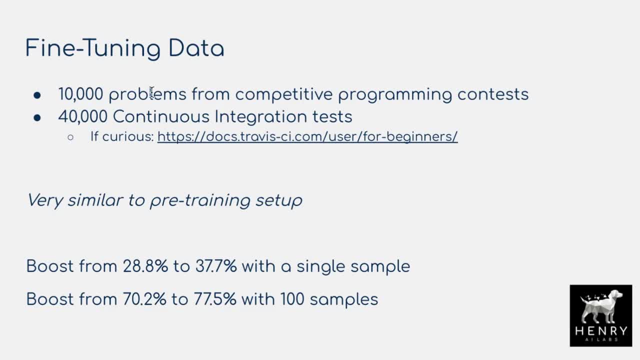 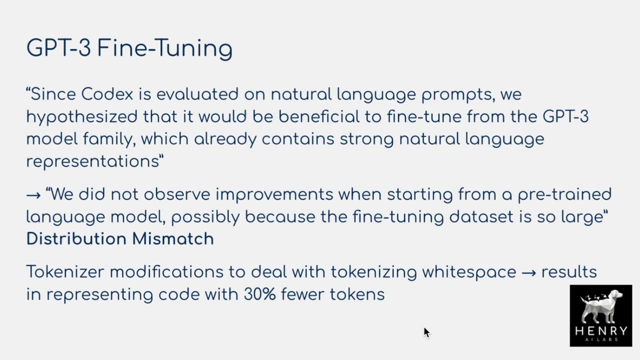 more domain relevant. So you're narrowing the distribution of the data to better align it with the downstream evaluation of, you know, solving these programming style questions. So the boost from doing this fine tuning is 28.8% to 37.7 with a single sample, 70 to 77 with 100 samples in the repeated sampling idea. So rather than starting training from scratch, the authors hypothesized that you could fine tune it from one of these GPT-3 checkpoints. So as they state, since Codex is evaluated on natural language prompts as in the doc strings or the, you know, the description of the programming, the interview style problem, we hypothesized that it would be beneficial to fine 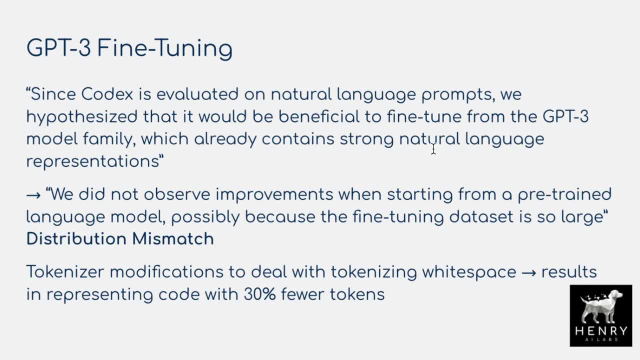 tune from the GPT-3 model family, which already contains strong natural language representations. But they find that this doesn't really improve the performance because the fine tuning data set is so 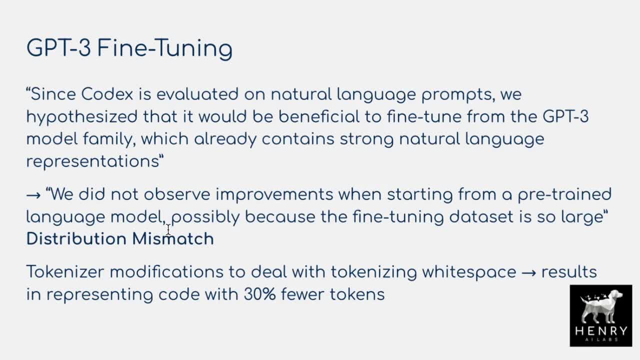 large. There's a distribution mismatch at the scale of 159 gigabytes of data. You don't need to do this fine tuning from the, you know, whatever GPT-3 was trained on. And they do describe that there's this tokenizer mismatch where GPT-3 is going to be able to do this fine tuning from the 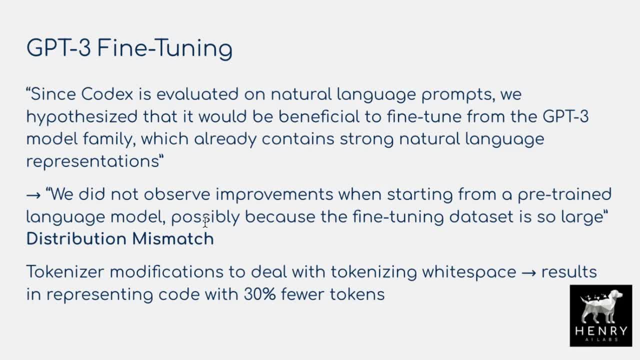 data set. And that's going to tokenize every whitespace token as a separate token. And that's going to result in a massive amount of blowing up the sequence length with code data because you 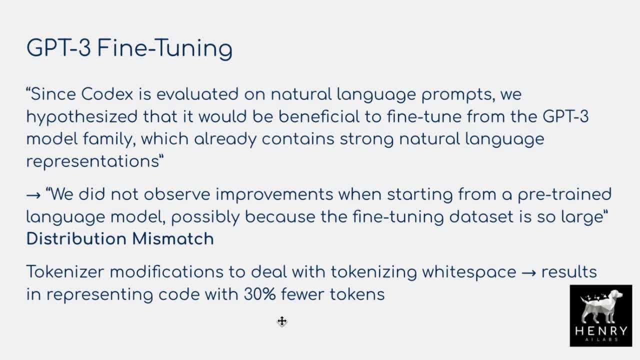 have a lot of whitespace with the way that you format code. So they use this little modification that results in representing code with 30% fewer tokens. So then they also pivot to the task of 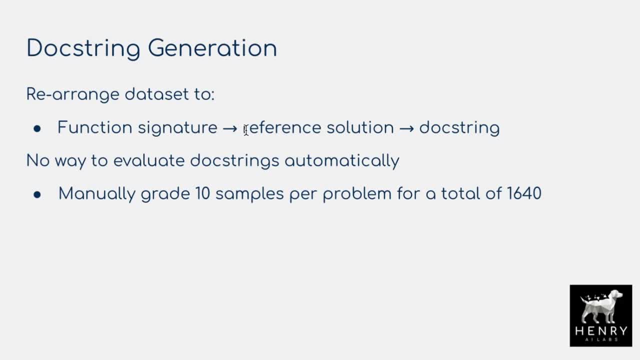 doc string string operation where you have the function signature and the solution and you want to generate some natural language description of the code. You want to have some, you know, language to describe what the code does. So the way they do this for fine tuning is they rearrange 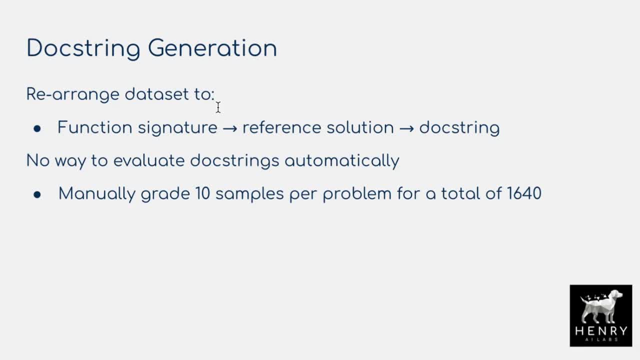 this data set. So instead of being, function signature doc string reference solution, it's going to be function signature reference solution doc string. So as you saw the previous examples of exactly what these look like, 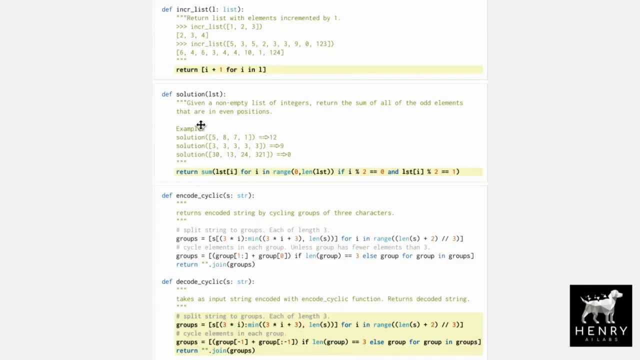 be, you know, instead of having this in the middle, this would be put at the end. And now this is the generation task that you use to fine tune the models to generate doc strings. And, you know, that that task, and it's hard to say whether this is harder than this or whatever, 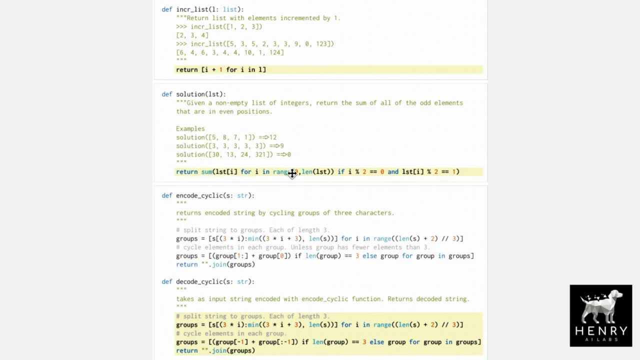 but, you know, it does seem like it's multi-line, maybe a little bit different in the way that it's done or multi-line, I don't know. But anyways, it's interesting to see this kind of difference 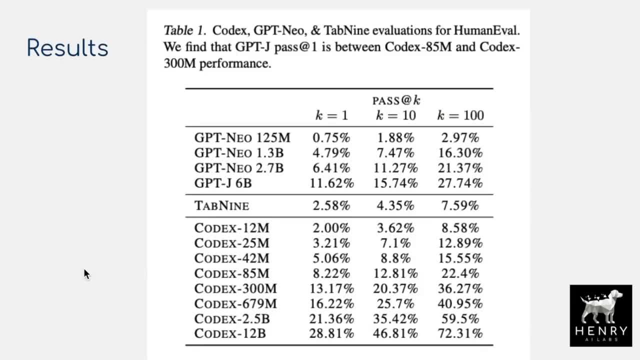 between generation and code generation. So here's the first table of results on this human eval data set, which again is 164 manually designed problems, each with about eight test cases. So they're 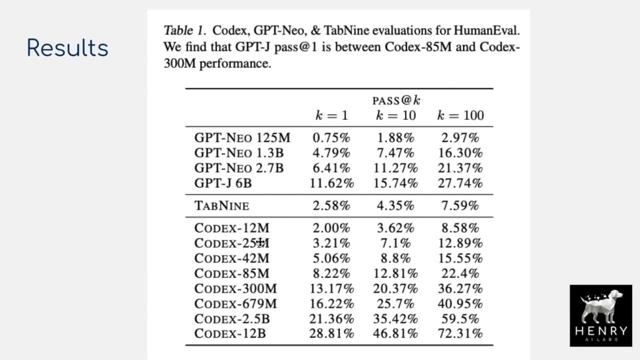 comparing the different scales of codecs going from 12 million, 25 million, 300 million, up to 12 billion, the passive K, this is how many repeated generations are used in order to get the winning 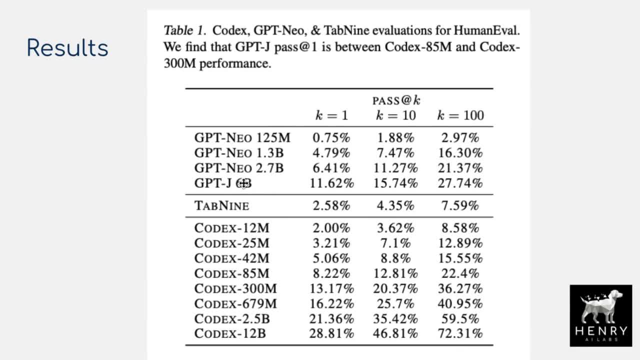 solution. And then comparing this with the GPT Neo models up to 6 billion parameters, as well as the commercial tab nine, 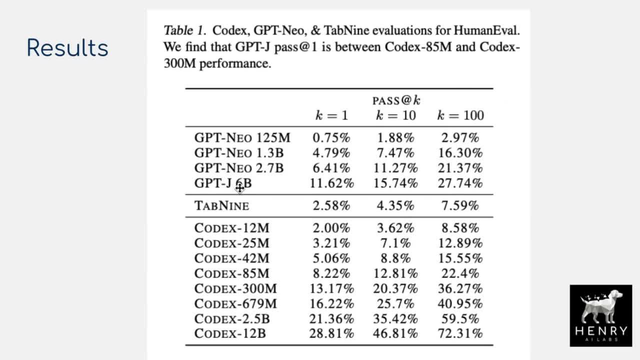 so they're showing that, you know, at 6 billion parameters, GPT J with 6 billion parameters is at 27.74, whereas codecs with 2.5 billion is, you know, about double that. So the GPT J, 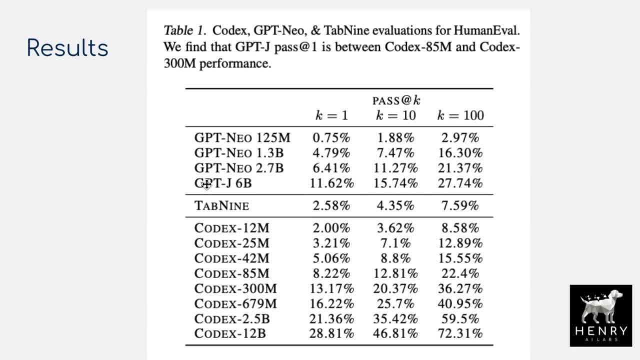 they describe their data set in the pile, Luther AI researchers. And this has, this does have some GitHub data, some stack overflow data. So it does have some code data. It's not like no code data is 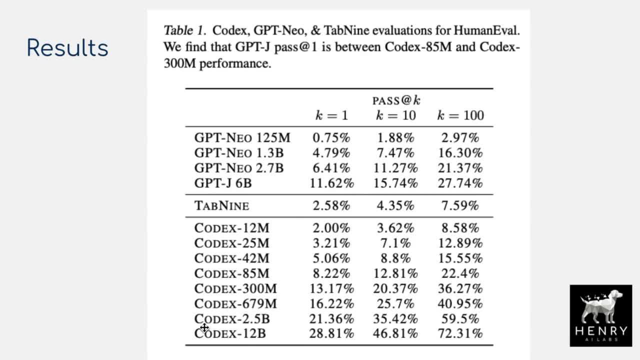 in it. And, but you know, this codecs thing, bigger data, GitHub, and so on. These aren't in the fine tune models yet. These are the just trained on the 159 gigabytes of data, not the 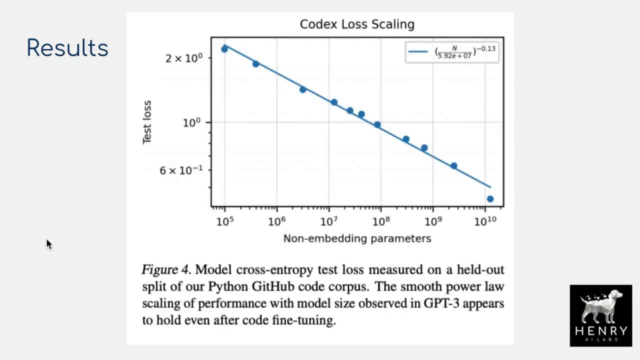 programming problems and the continuous integration tests. So also in the trend of scaling up the model size, we've seen tons of these papers that are looking at the scaling laws. And you know, giving us some equation like this, we've seen it for, you know, neural scaling laws, these autoregressive language models, autoregressive generation, and so on, where you show that 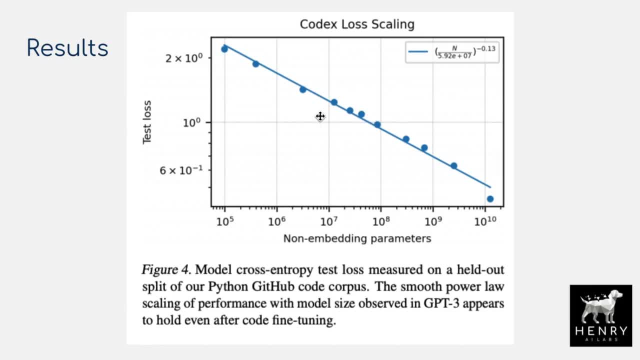 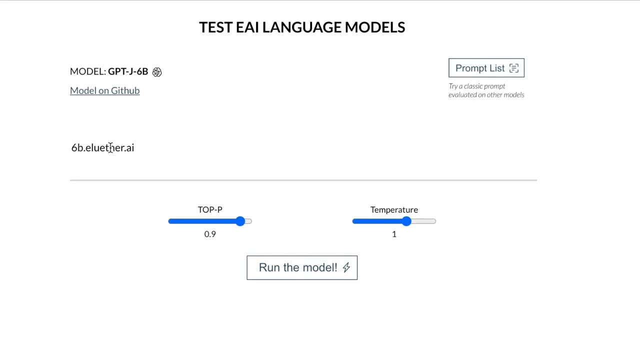 basically, you increase it by 10x to kind of move along the y axis a little bit. So this is showing the codecs models from say, you know, 100 million parameters to a billion parameters and so on. So if you want to play around with the GPT Neo models, here is a demo hosted on 6b.luther.ai, you can put 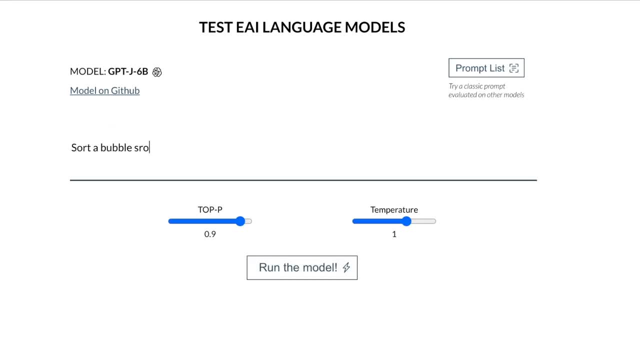 in whatever prompt you want, like, you know, sort of bubble list with Python or a bubble sort of list of Python or, you know, reverse a binary tree, whatever with these kinds of these are the kinds of programming problems that we're talking about, you can test around with these prompts, if you 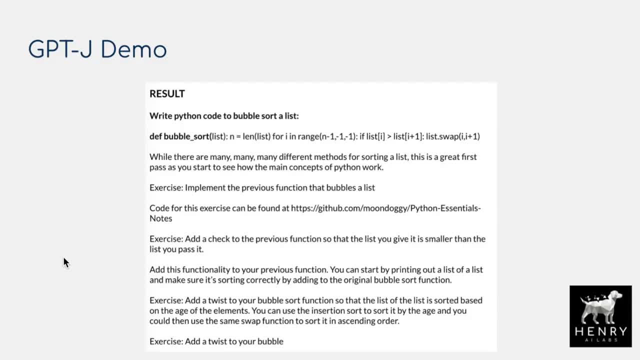 want to, you know, play around with this model and see what it'll generate. So here's a quick look at the render demo, if you give it something like write Python code to bubble sort of list, death bubble sort, and then you let it, you know, finish it, it'll do the correct style of Python list, 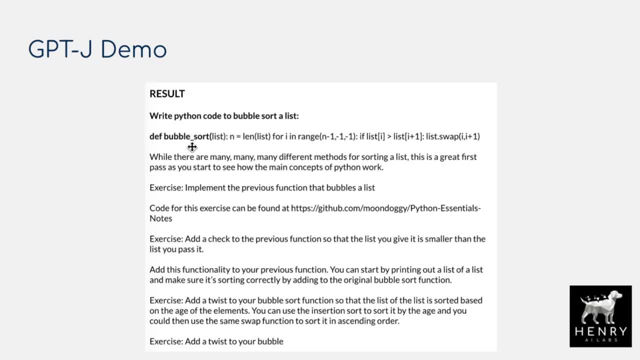 you know, it doesn't do like the indent thing, I don't know if it would have to do like new line, and then tab and so on to, you know, simulate the Python syntax. But you see, it has some understanding of looping through this list doing some kind of comparison, then swapping the elements, 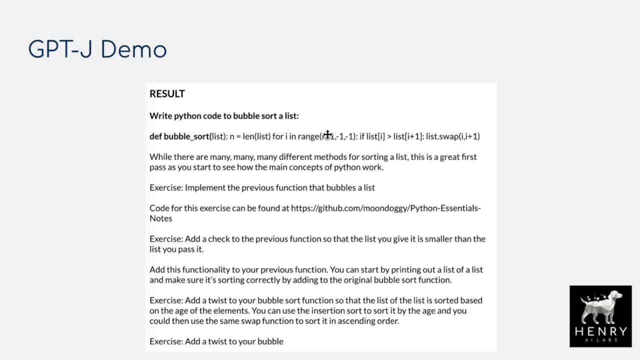 the kind of bubble sort idea, it doesn't look to be like exactly correct with the way it sets up the range. And then you know, there are more description as you keep generating with the model 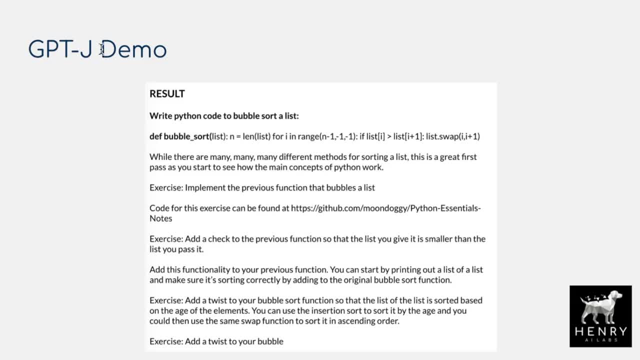 and keep going into the generation tree. So it's really interesting and fun to play around with this GPT J demo that makes it so you know, anyone can get a sense of what's going on with these large 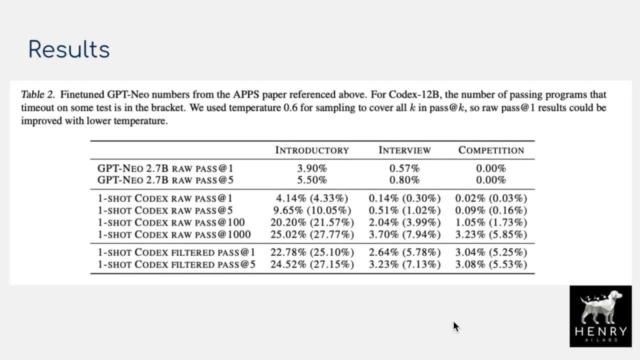 scale language models. So in addition to the manually constructed human eval data set with 164 examples, they also evaluated on the apps challenge. So the apps challenge, it's also from 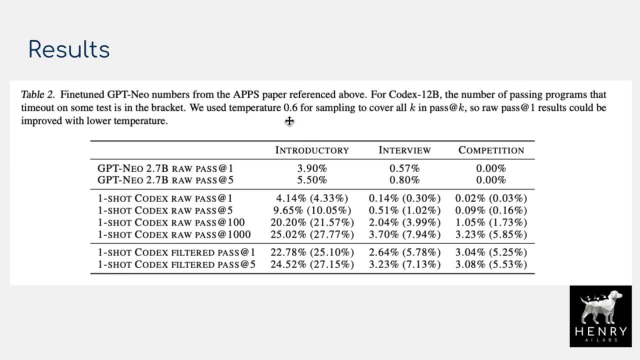 code forces, these different interview styles, introductory, not also human eval is not from that. 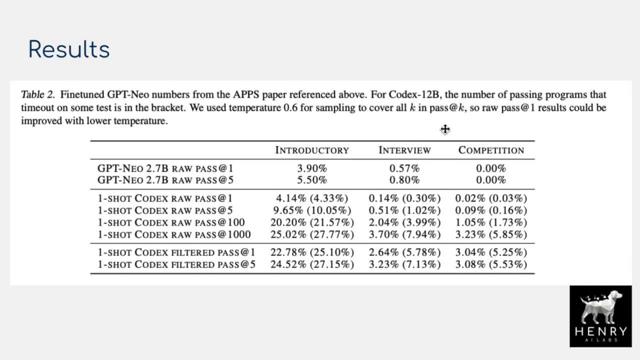 But anyways, so they have these different categories, introductory interview competition, the different levels of difficulty of the challenges. 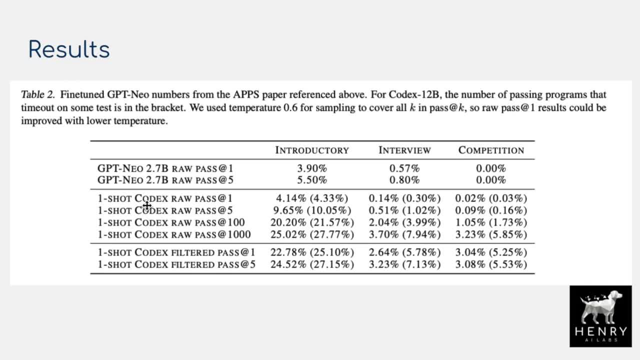 And these are the one shot results of codecs, codecs, comparing it with the raw unfiltered pass. I'm not I don't exactly remember why that is. But you know, the passive one 500 1000 thing as you 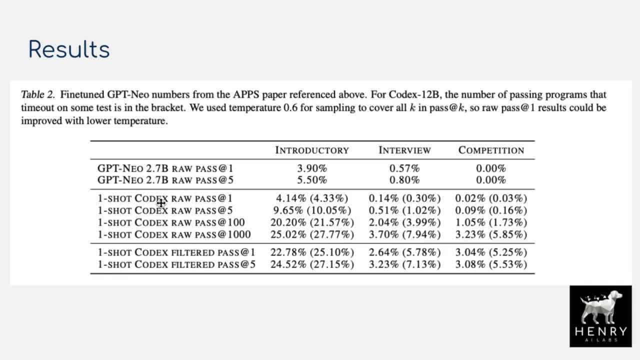 increase the number of samples generated, and then one shot meaning that this hasn't been fine tuned yet. And you're using some kind of demonstration of a programming problem in the context window of 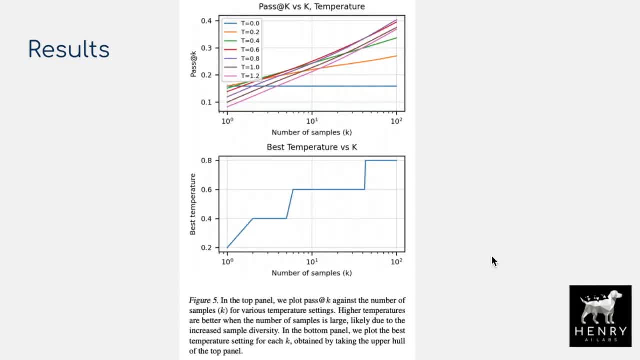 the language model. So here's some more plots digging further into the results. This is where they're plotting the number of samples k and then the temperature temperature is a hyper parameter 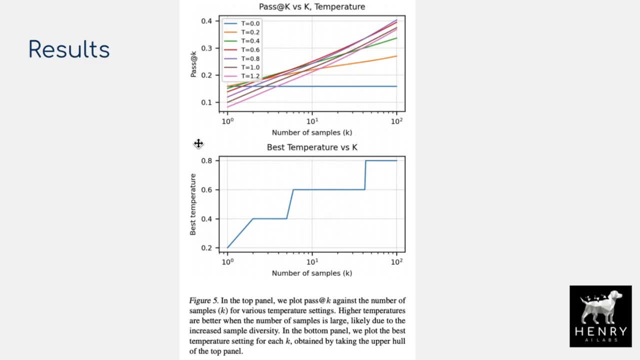 distribution, looking at the optimal value to use for this temperature, probably something to do with the way that you smooth out the logits where you have like the exponential the logic divided by 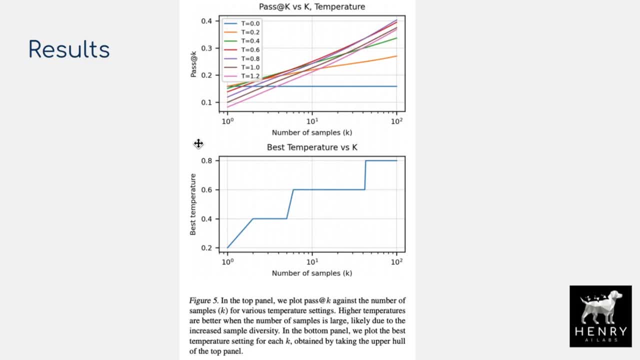 the temperature with respect to how you form that probability distribution for the next token. This is showing the pass rate versus the model size, showing an interesting thing about this plot is 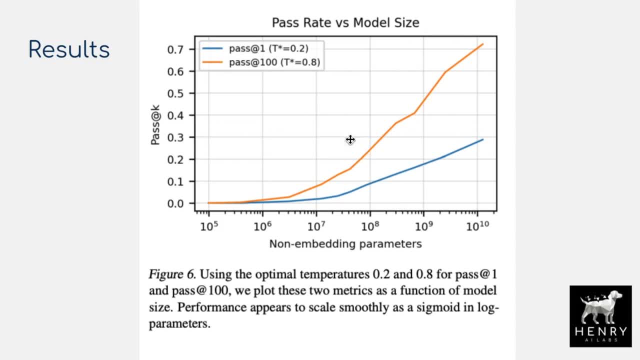 that they show that you know, as you are doing more generations to the passive 100. Now it benefits to have a higher temperature parameter. So you have 0.8, which means it has more 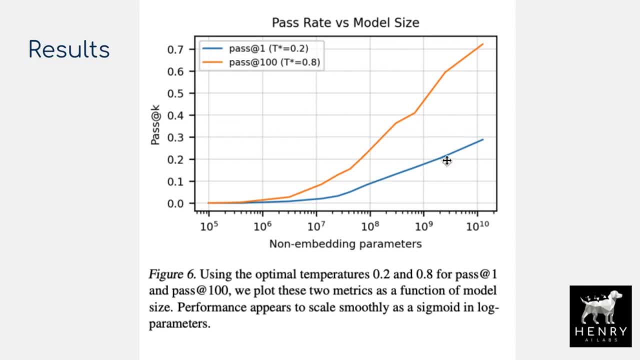 solutions. And then this also continues to be the case as you increase the number of parameters to 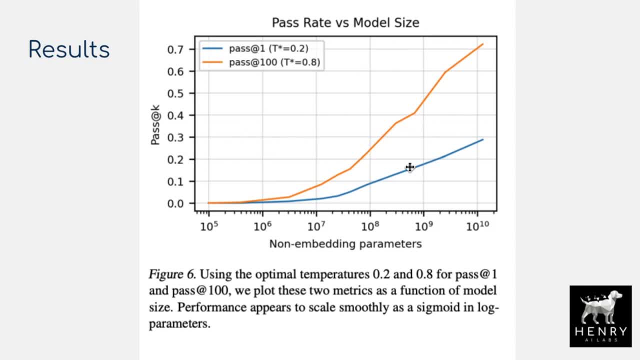 say a higher capacity model knows how to do more diverse generations, or knows it has it in the parameters of the model. And then then the temperature thing is how you kind of probe for 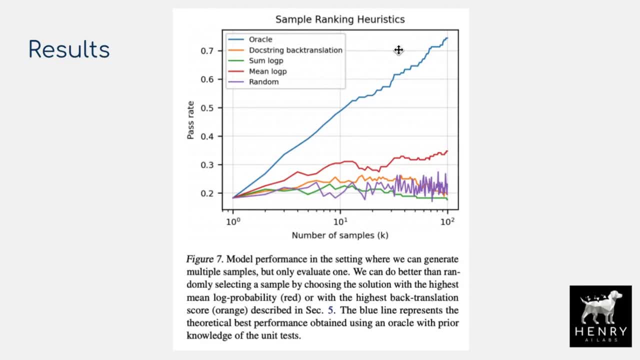 that. So then simple ranking heuristics. So you know, you're generating 100 1000 samples, how are 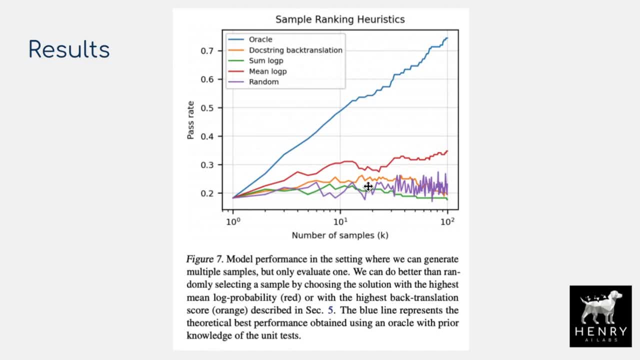 you going to rank them, they use the doc string thing that uses back translation between the 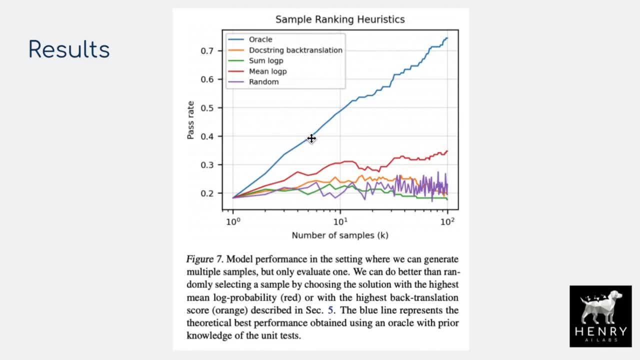 generated and original doc string is one way of ranking this. When you do the mean log probability, this is where you, you know, take the average of the 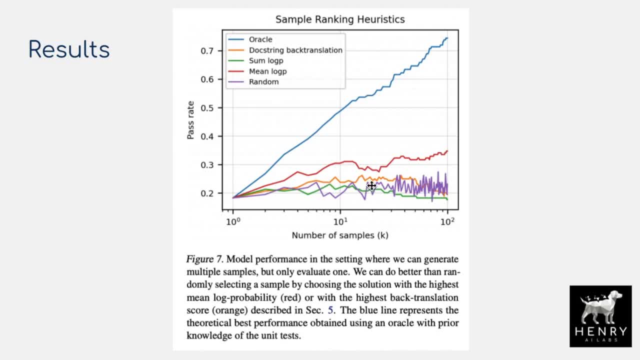 probabilities as you go through the tree compared to say summing them up, kind of surprising that 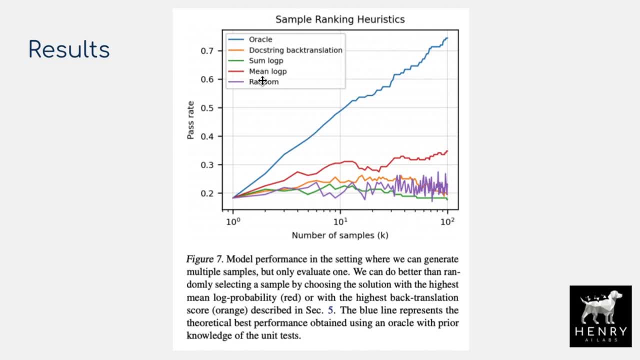 you know, the mean is performing so much better than summing them up, but and then just random 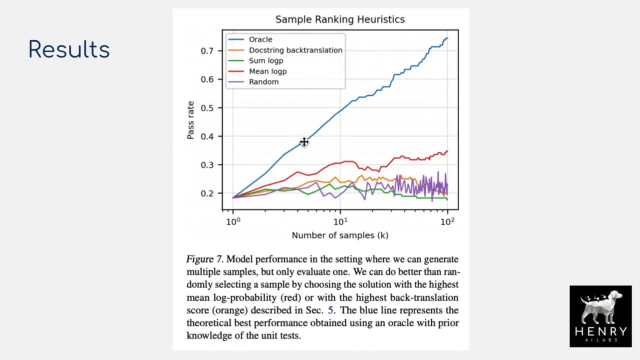 selection for which one of the 100 generations are, you know, given to the unit test and that 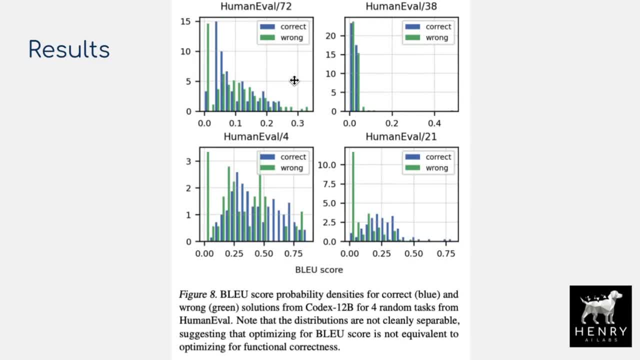 kind of idea. So this is also showing this problem with the blue score, this is one of the most 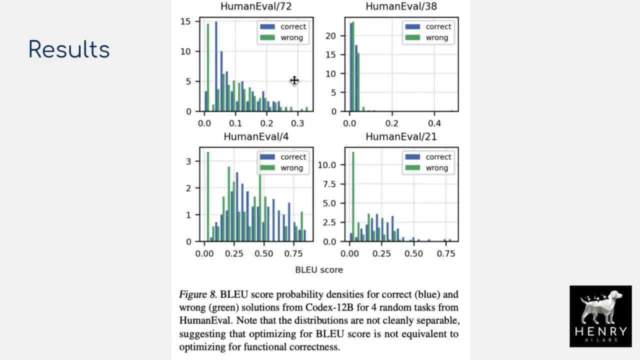 interesting trends of this research, I in my opinion, is that the you know, you have this 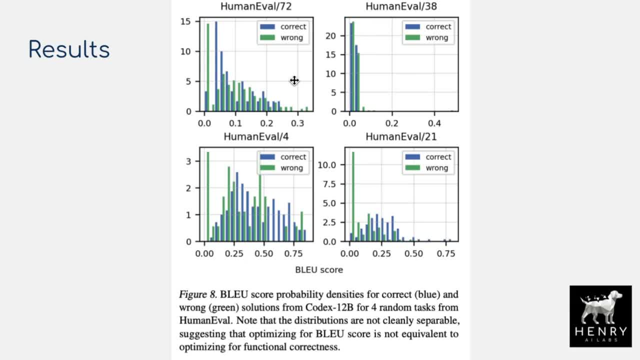 unit test ground truth evaluation thing, compared to these other kind of heuristic evaluations they 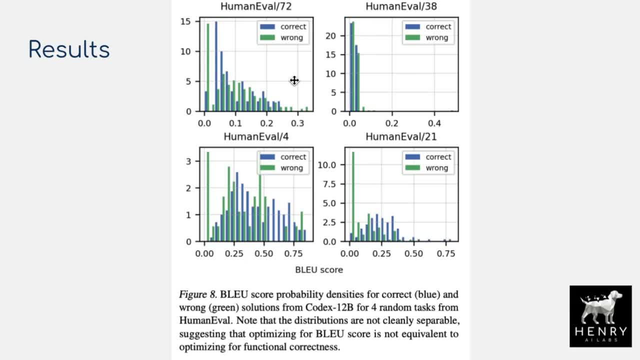 use. So blue score is like a matching metric. So you have this ground, say it's abstractive 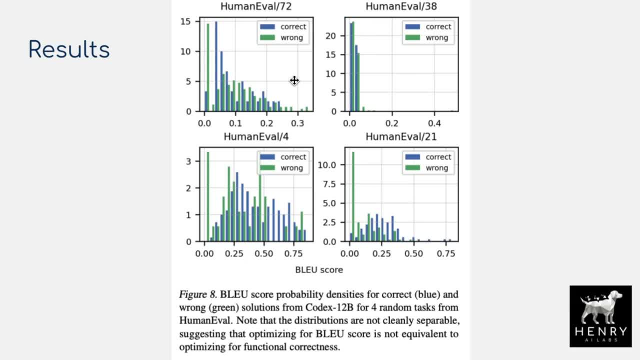 optimization, and you have some kind of ground truth summary of a reference article, you'll you'll 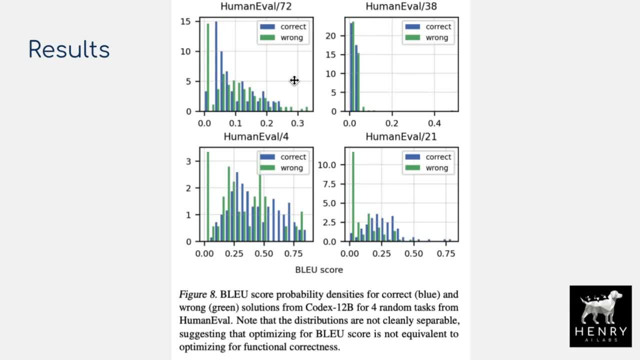 measure the output of the model by how well it matches exactly the ground truth thing. So when 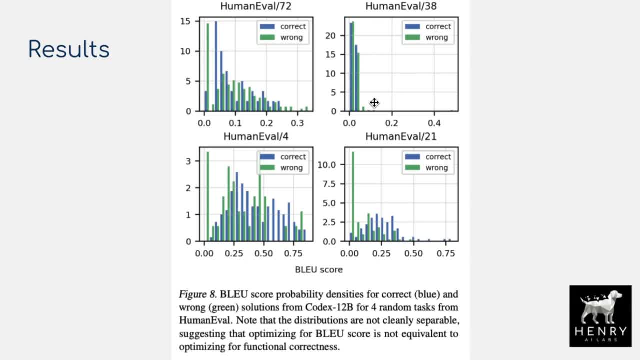 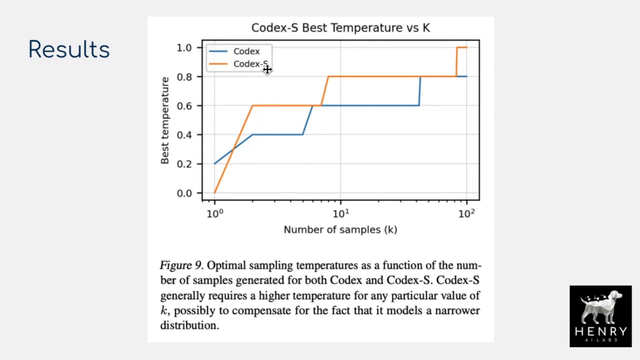 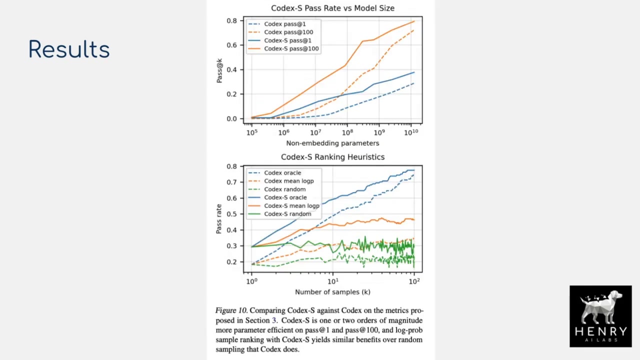 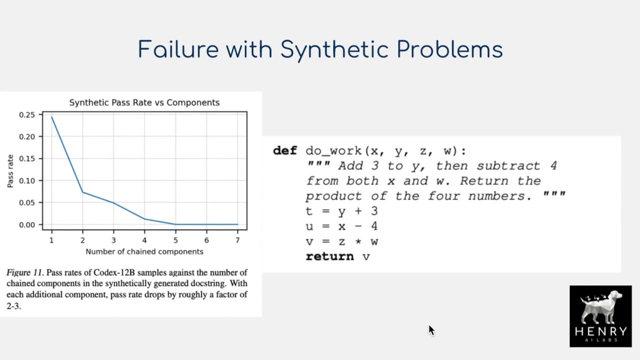 you use the exact ground truth of the reference, you know, programs, then you get a high overlap locking score, but they might not have the same functional equivalence, and so on and not pass the test. So they're showing that, you know, higher blue score doesn't necessarily lead to, you know, better unit test passing, it's just the fundamental problem of evaluating these text generation models automatically. And then this is showing, you know, again, the fine tune model, the Codex S is fine tuned on the 10,000 programming problems, 40,000 continuous integration tests, compared with the non fine tune model. And then also looking at that same kind of trend, but with respect to model size, and then more on the ranking heuristics on how you can try to sample one without, you know, without having to just generate 1000 of them and so on. So they further do some qualitative analysis of where the model is failing, they have these artificially constructed tests where they chain together different things, like add these two numbers, then, you know, say you add three to y, and then just kind of chain that over and over again, and go, say, then subtract four from y, then multiply y by eight, you do these long chain chains. And this is where the model will start to break down. And it also shows that, 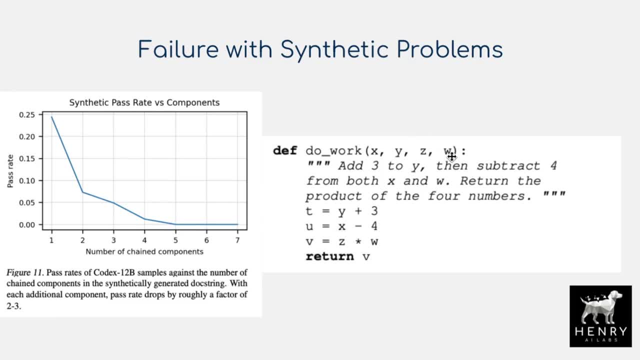 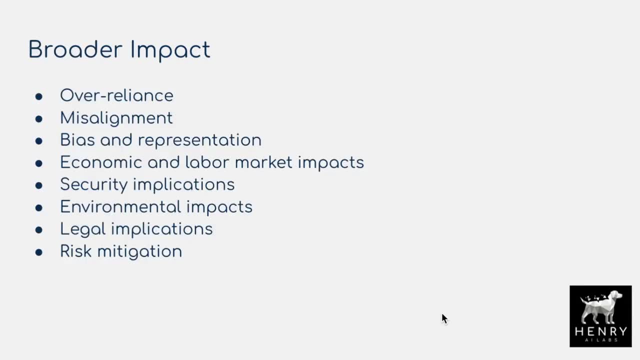 you know, it breaks down with this idea of variable binding, and being consistent with, you know, using the variables to, you know, do these sequences of calculations as shown here. So as this idea of deep learning with code data, and these artificial intelligence deep neural network models 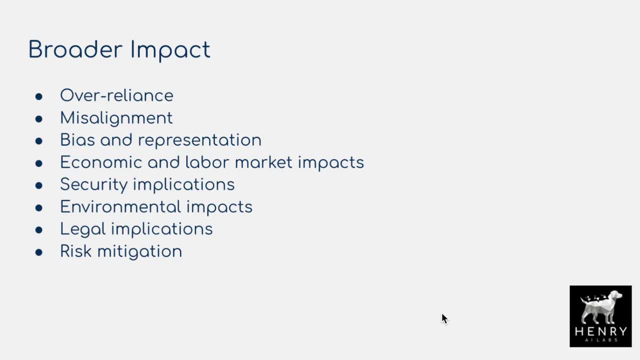 that can write code, I think that's a really good idea. And then, you know, if you're not familiar with the AI team, 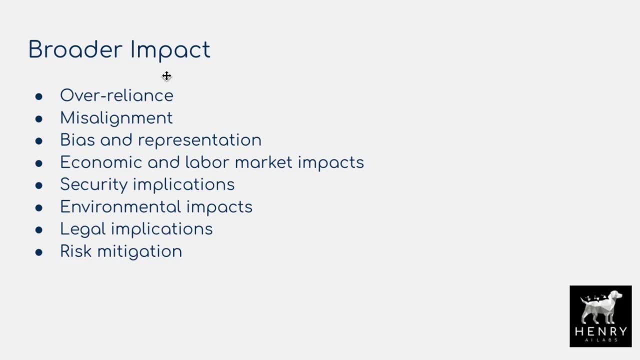 there's a really great policy team that is kind of analyzing the impact of what this technology might do. And their broader impact statement, they described the over reliance as programmers may 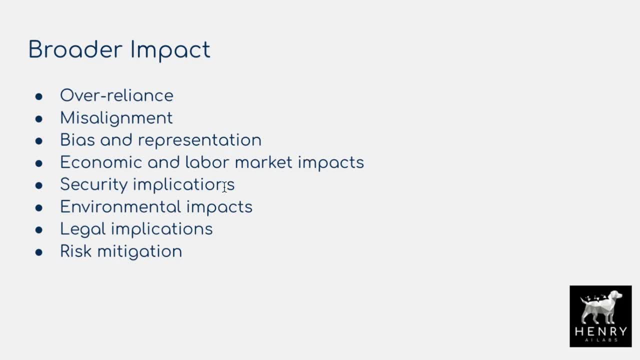 over rely on these models, and that kind of idea, misalignment, bias and representation, economic and labor market impacts, security implications, environmental impacts, legal implications, this 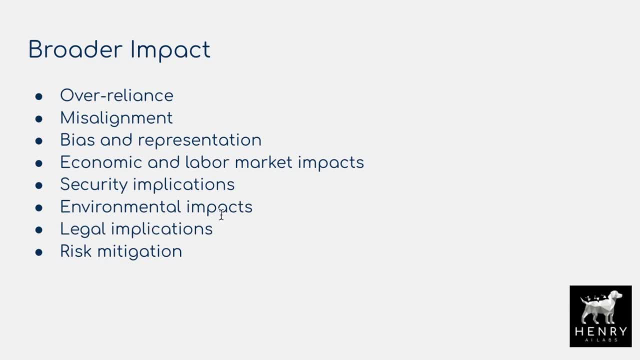 has been a big one I've seen on Twitter, where people are like finding their code, it's not, you know, looking at the licenses of these public repositories, and so on. And then risk mitigation. So I hope that's a good idea.